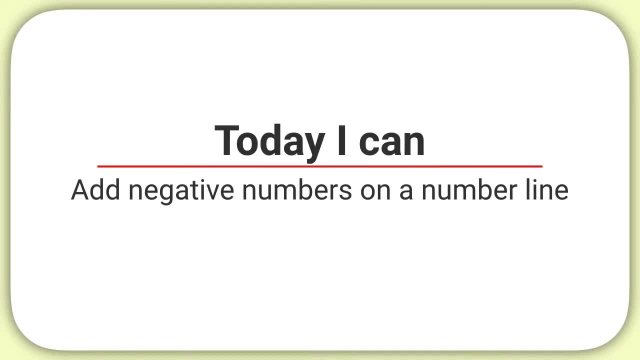 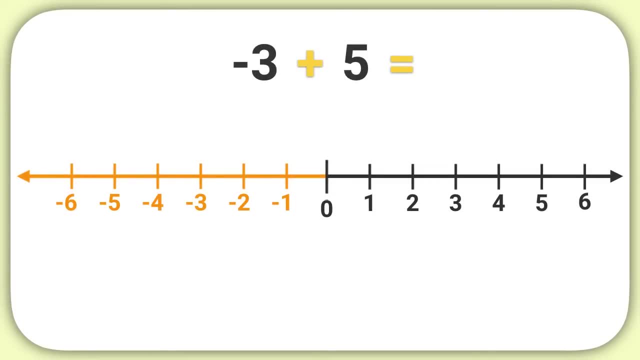 Today we are learning how to add negative numbers on a number line. Let's say we wanted to add negative 3 plus 5.. We'll start at negative 3 and we'll draw a person right there Now because we are adding. this person is facing forward on the number line To add 5, that person will walk. 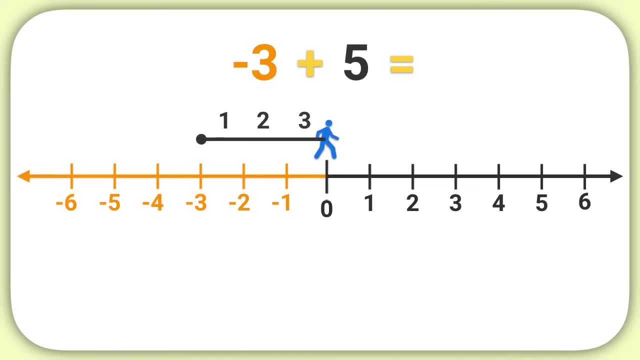 forward: one space, two spaces, three spaces, four spaces, five spaces. Now we can see the person is at 2.. So negative 3 plus 5 is 2.. Let's look at another problem, though Let's figure out what 4. 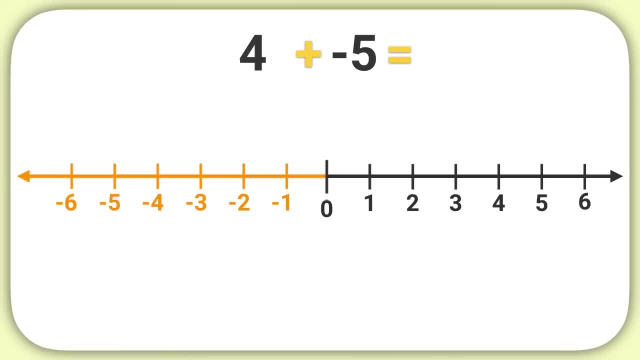 plus negative 5 equals. This time we're starting with 4.. We'll draw our person at 4,, but we're adding a negative 5.. Because we are adding a negative number, our person is not going to walk forward. They're going to walk backwards five spaces. We'll walk backwards one space, two. 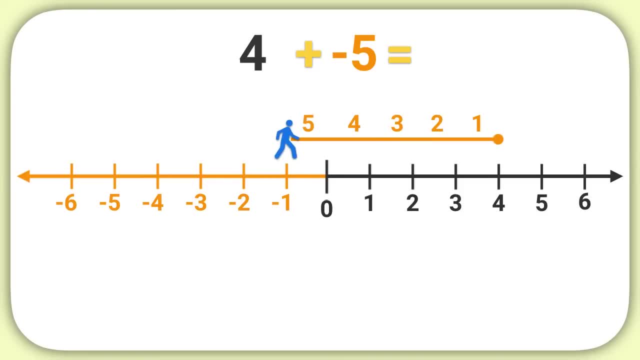 spaces, three spaces, four spaces. Now we can see that the person is facing forward one space, three spaces, four spaces, five spaces. Now we can see our person is at negative 1.. So 4 plus negative 5 is equal to negative 1.. Now it's time for us to practice together. Let's figure out. 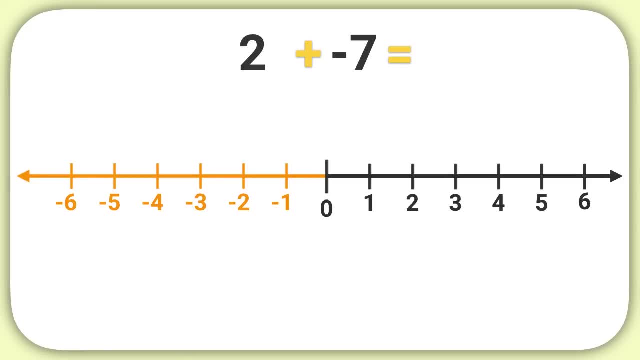 what 2 plus negative 7 is. Well, I'll start at the number 2.. Then I need to add negative 7.. When I add a negative number, am I moving forward or backwards on the number line? When I'm adding a negative number, I move backwards. I'll move backwards one space, two spaces. 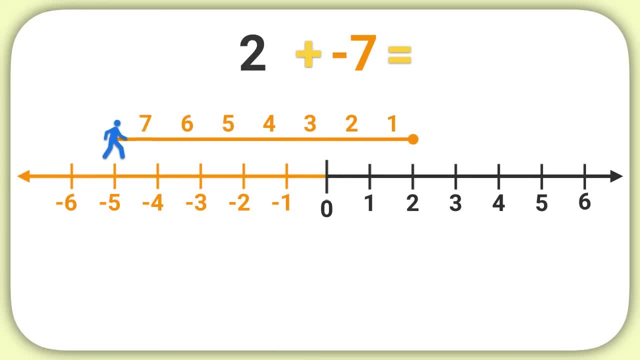 3, 4,, 5, 6, 7.. So what is 2 plus negative 7?? Well, now we're at negative 5.. So the answer is negative 5.. Here's another problem to practice with. Let's add negative 6 plus 4.. Well, 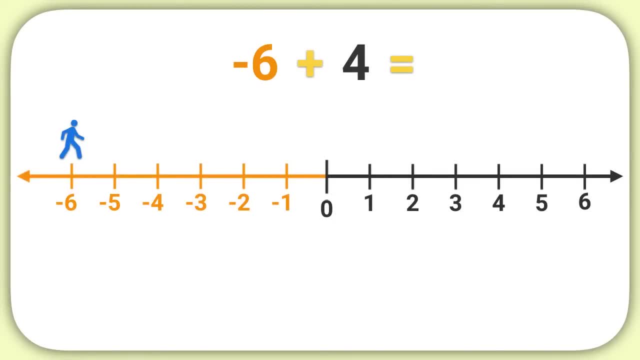 I'm going to start at negative 6 on my number line. Then what should I do? Well, I'm adding positive 4.. So I'm adding a positive number. My person is going to walk forwards. If I walk forwards four spaces, where on the number line will I be? Well, if I move forward one space,